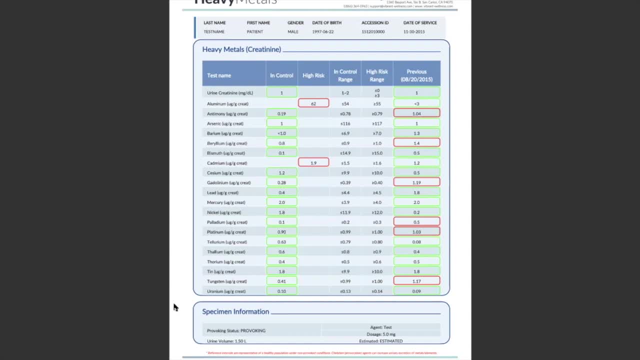 they can accumulate in air, soil and water sources, so this would be valid in every area of the country. Heavy metal toxicity is underrepresented as a root cause of illness and disease in humans and can affect virtually all biological systems within the body. Heavy metals may be the root cause of common neurological disorders, making this a great 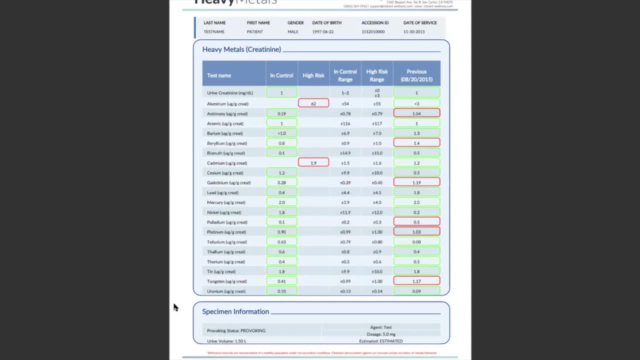 pairing with our NeuroZoomer or NeuroZoomer Plus. Also, heavy metals may be causing gastrointestinal disorders, such as they can deplete levels of beneficial flora and promote growth of resistant bacteria associated with IBS and SIBO, and can also be a cause of intestinal permeability. So this would also be a great test to run alongside. 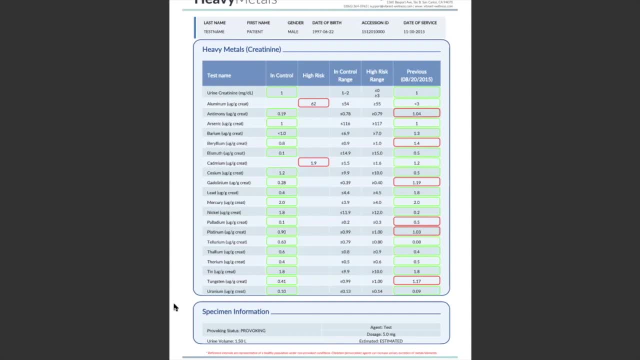 a gut zoomer. Other disorders associated include increased oxidative stress and cellular dysfunction. So, due to the ability of many heavy metals to deplete critical nutrients such as antioxidants and minerals, the vibrant heavy metals test should always be run alongside a vibrant micronutrient panel to assess intra and extracellular as well as red blood cell levels. 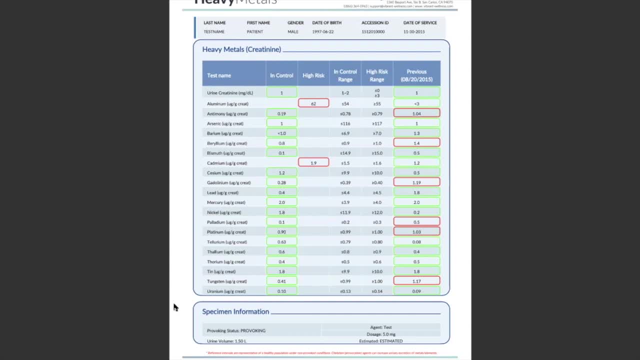 of commonly affected nutrients. Along with our heavy metals guy um heavy metals test, we also provide blood cell and red blood cells and we also provide blood cell and blood cell and We have a companion guide and I'm going to show you that. 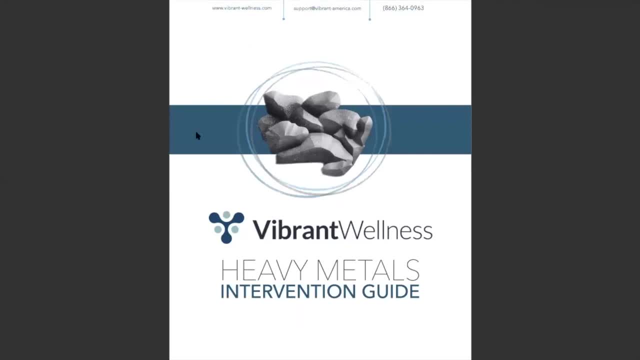 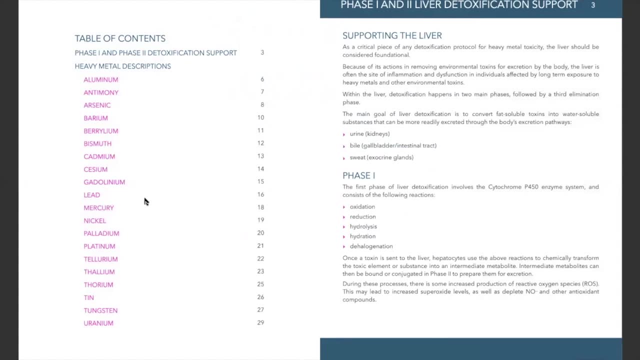 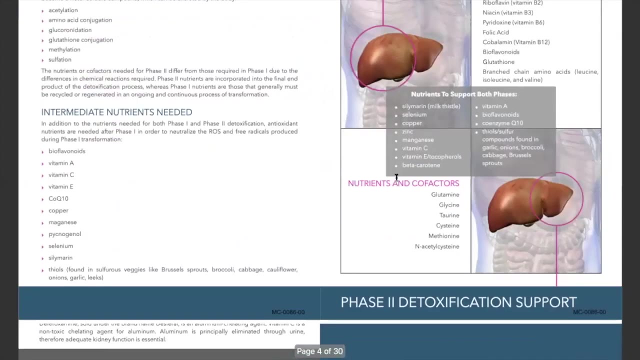 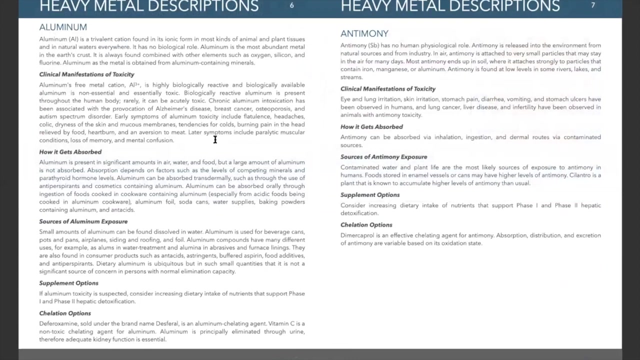 So here we have our heavy metals guide, intervention guide, and you can see we have a listing the table of contents of all the different metals and then some liver detoxification support information And then for each metal we're listing information about the metal: clinical manifestations of toxicity, how it gets absorbed, sources of exposure, supplement options and chelation options. 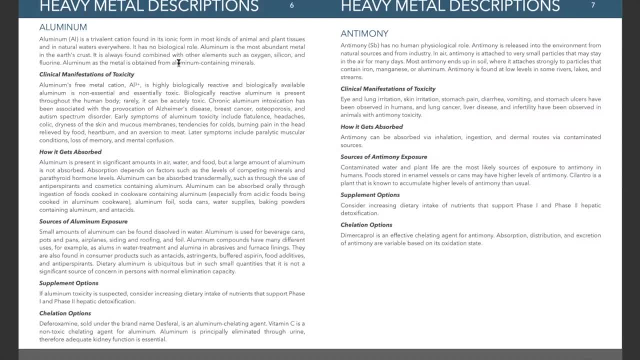 So, along with your heavy metals test, we have a companion guide, so you will have all the information you need to be able to use this alongside of your other Vibrant Wellness testing. Thank you so much. Thank you for your attention and let us know if we can answer any other questions. Thank you.